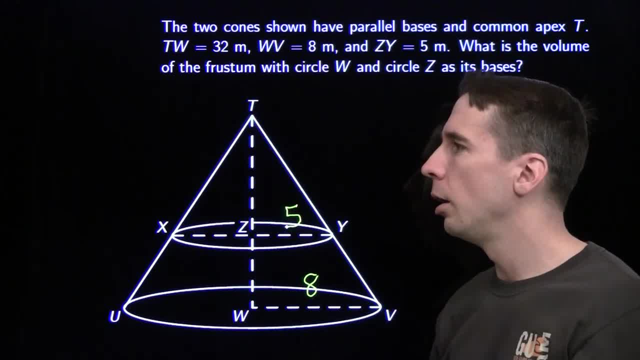 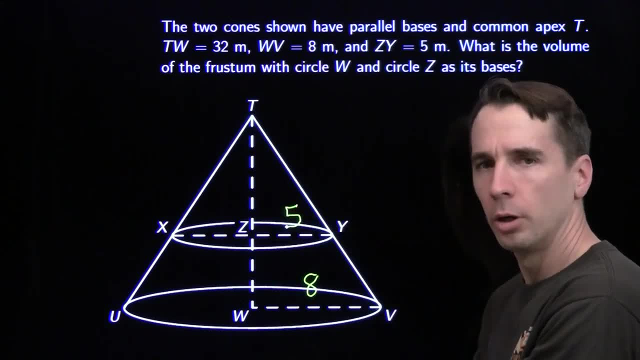 so this height is 4 times this radius, so this height is 20, da-da-da-da-da. Oh, okay, You're right, We didn't need to do all that because, well, we know, these two cones are similar. 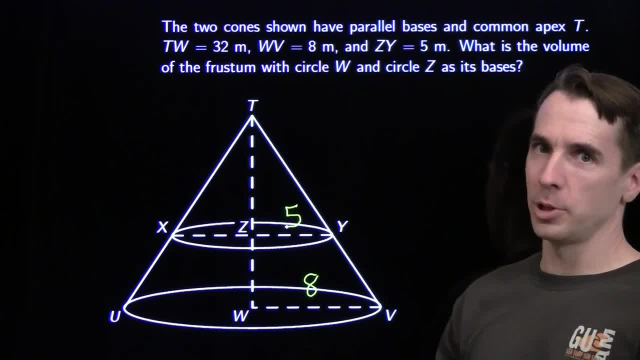 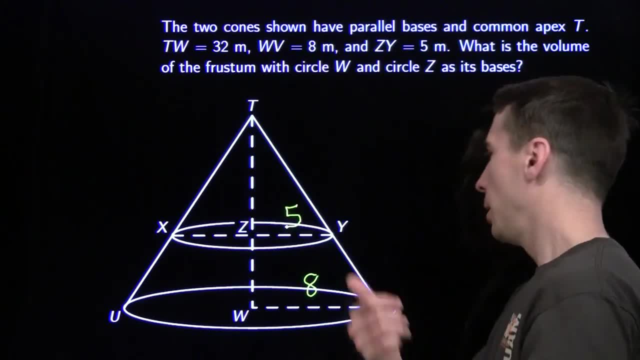 and we know the ratio of the corresponding sides, so we know the ratio of the corresponding volumes. This radius is 5 eighths This radius, so the volume of the little cone is the cube of 5 eighths times the volume of the large cone. 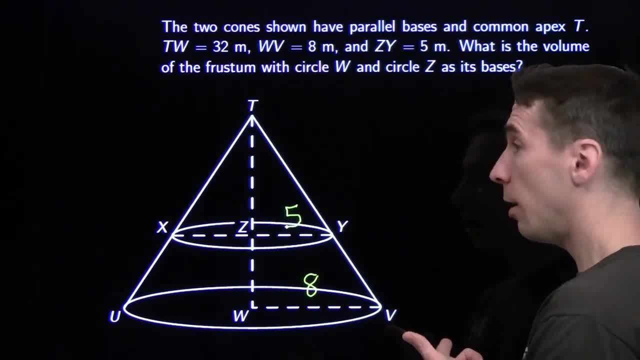 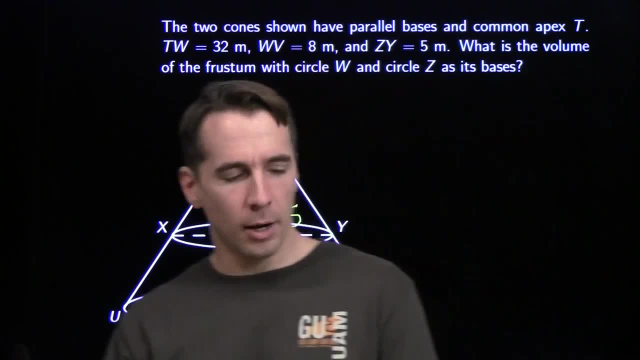 And now the problem is just arithmetic. You want to knock off the honors Because I'm not left-handed. No, You don't do arithmetic. All right, Step over here, Harvey, Get out of the way. Oh, come on. come on, Get out of the way so they can see it. 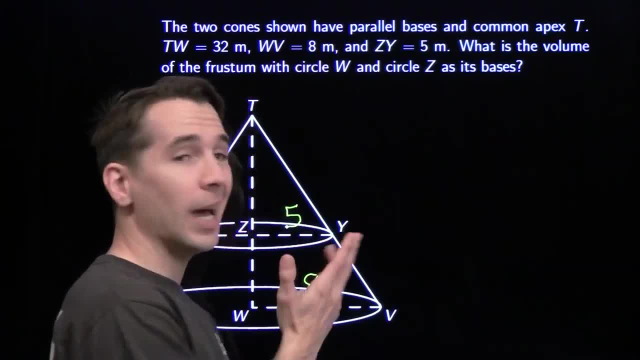 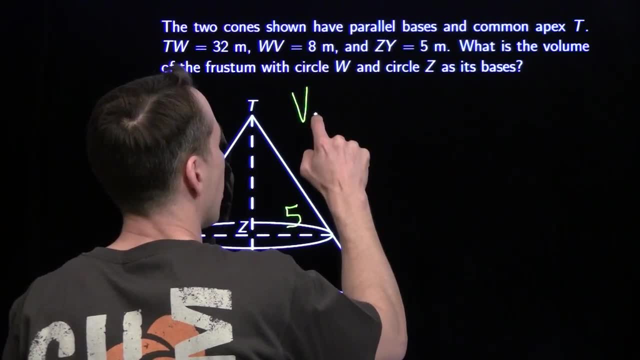 All right, Good, All right. I'll take care of the arithmetic, because you know what having a great idea is only half the battle. You also have to have good execution, So let's take care of this. Our strategy is to start with the volume of the big cone, subtract the volume of the small cone. 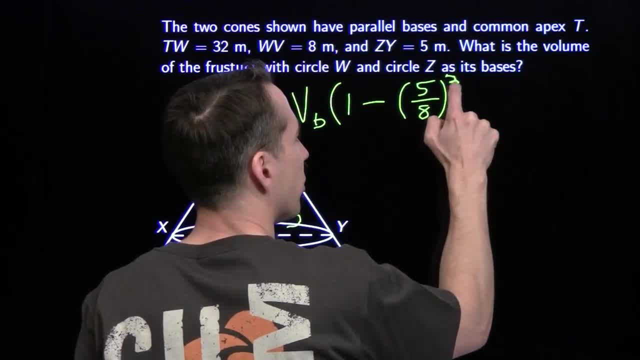 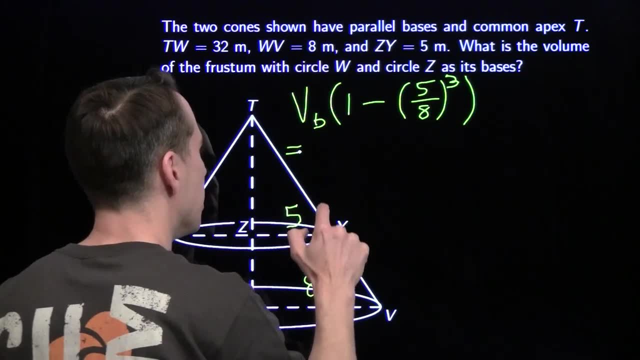 The small cone is the cube of 5 eighths. So 5 eighths times the large cone, That's its volume. So there's our strategy: Volume of the big cone minus volume of the small cone. Volume of the big cone: we know its dimensions, so we can crank that out. 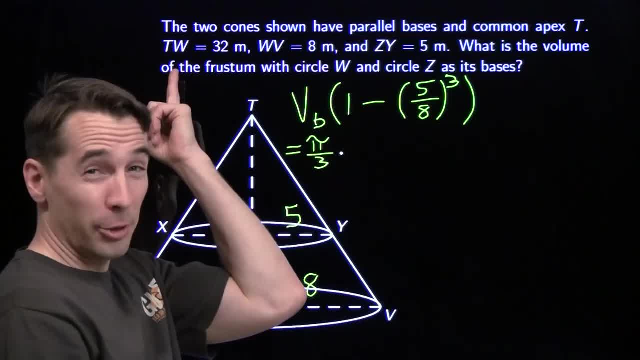 It's 1 third of pi times the radius, So the radius there 32.. I'm going to write that down as 2 to the fifth because I see that 8 sitting there, I know I'm going to get some cancellation down the line. 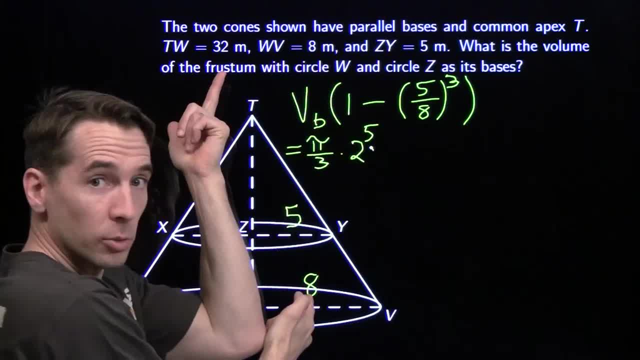 We write that as 2 to the fifth And then we have to square the radius. The radius is 8.. Another power of 2. That's 2 cubed. Square 2 cubed, you get 2 to the sixth. 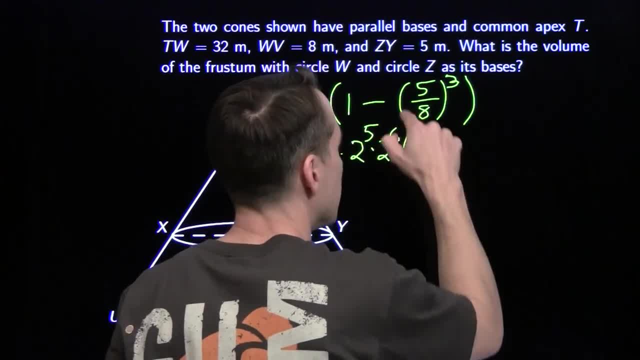 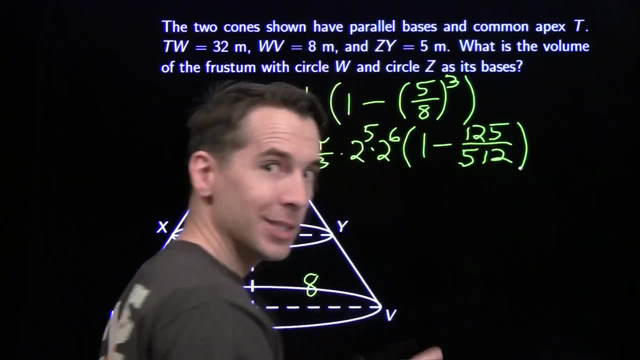 And then we've got to do some arithmetic. We cube 5, we get 125.. We cube 8, we get 512. Those two numbers have the same digits in different orders. Total coincidence. but I like geeking out over numbers like that. 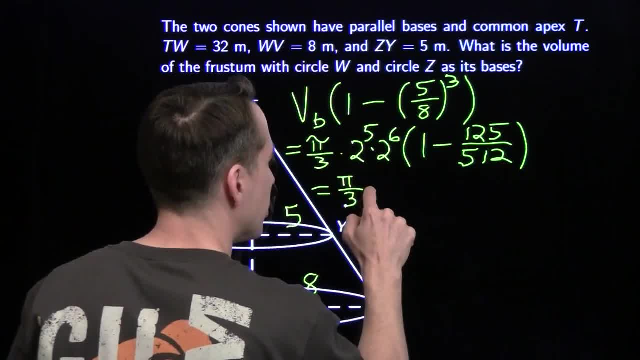 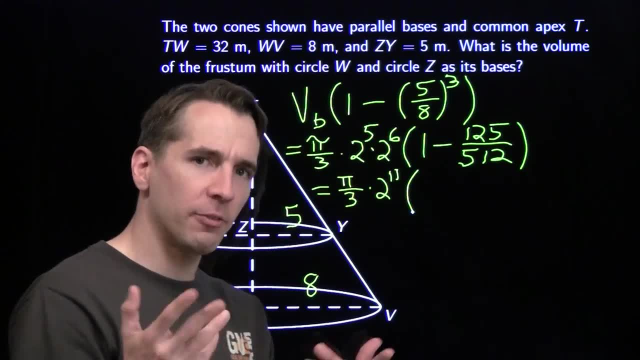 And now let's finish our arithmetic. 2 to the fifth times 2 to the sixth, that gives us 2 to the eleventh. Now that 1 there. we can think of that as 512 over 512.. Subtract 125 from 512, you get 387.. 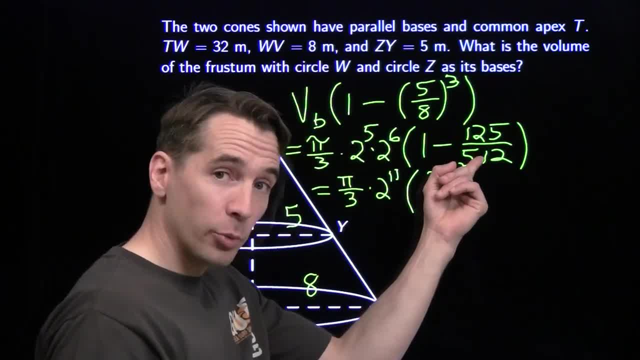 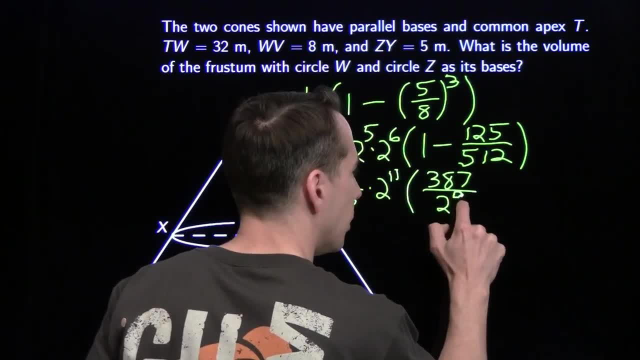 Now we've lined up that cancellation here, so I'm going to take that 5 to the twelfth and think of it as a power of 2.. That's 2 to the ninth. 8 is 2 cubed. You cube 2 cubed. you get 2 to the ninth. 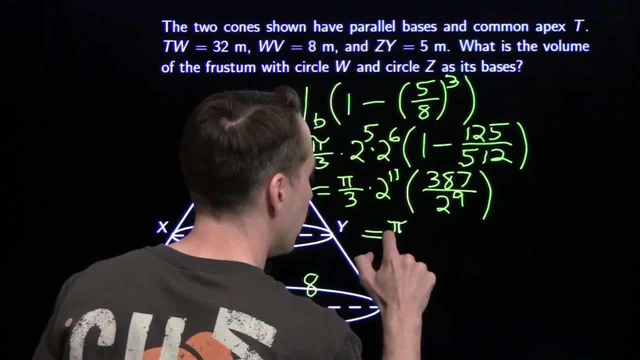 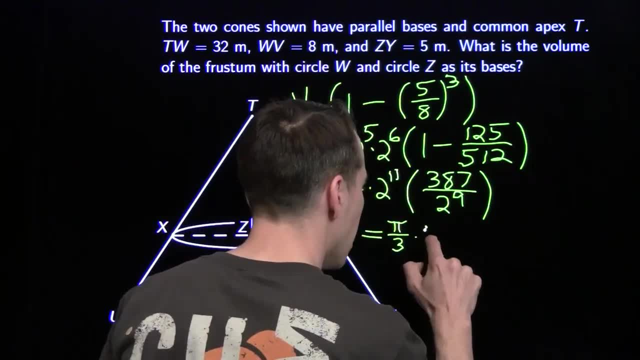 And now we've got that cancellation all lined up, We have still that pi over 3 times 2 to the eleventh, divided by 2 to the ninth, That gives us 2 squared. 2 squared otherwise known as 4 times 387.. 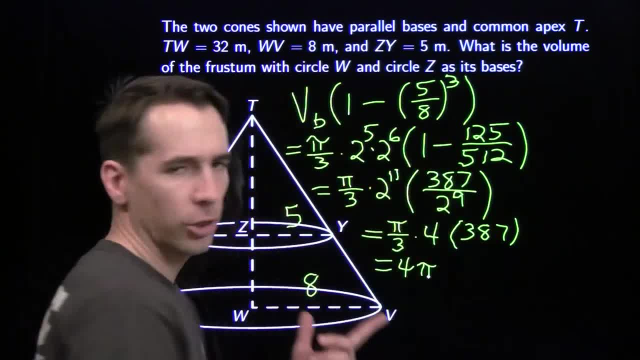 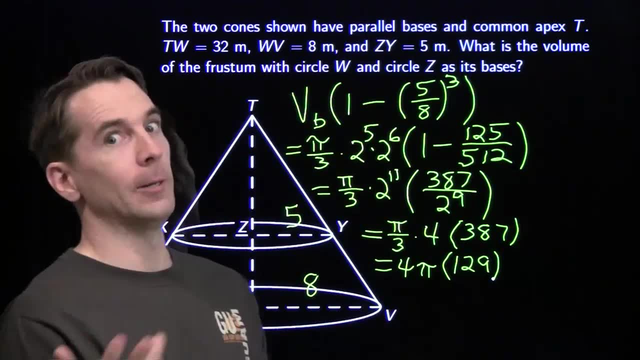 Well, now I've got 4 pi sitting out here. When I divide 3 into 387, I'm going to get 129.. If you don't see that right away, you can think of 387 as 390 minus 3.. 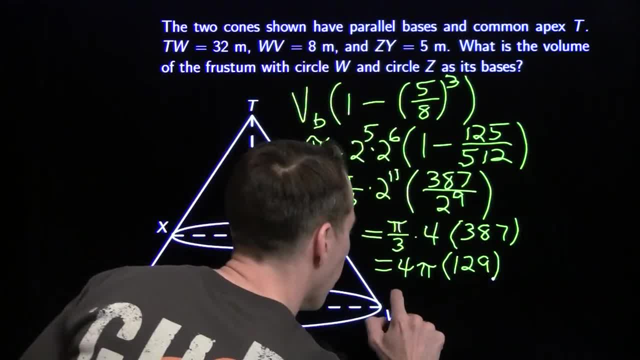 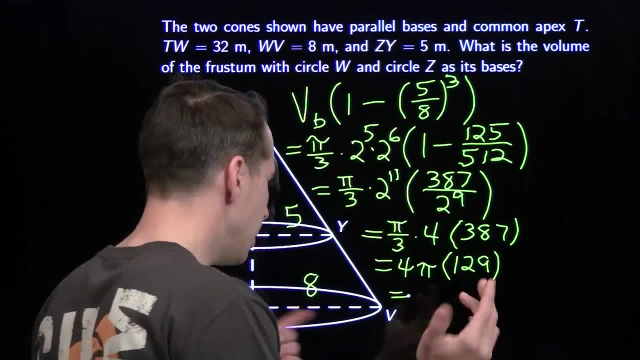 Divide 390 by 3, you get 130.. Divide 3 by 3, you get 1.. You get 429. when you subtract Now 4 pi times 129.. 4 times 125 is 500.. 4 times 4 is 16.. 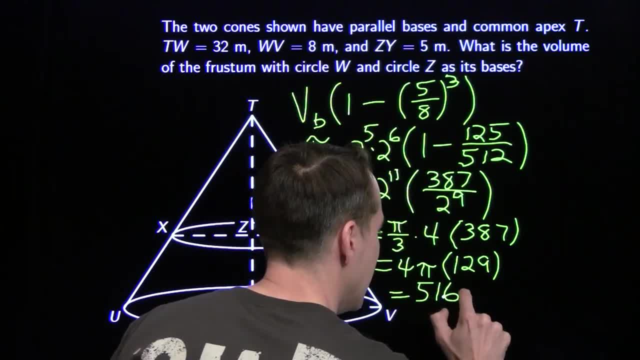 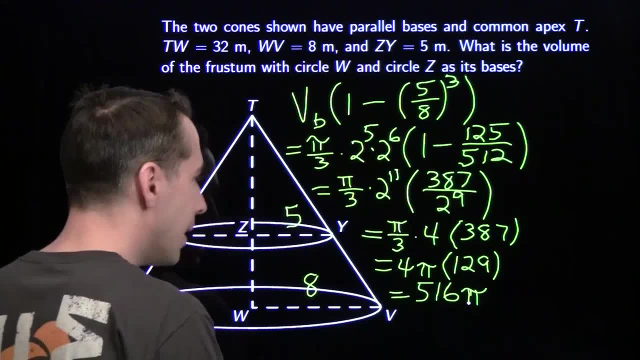 500 plus 16 is 516 to go with our pi. All right, there you go. There's the execution. Harvey, you can dial it back in now because we're finished with the arithmetic and we've answered our problem. So to take away from this, you remember we've got a frustum. 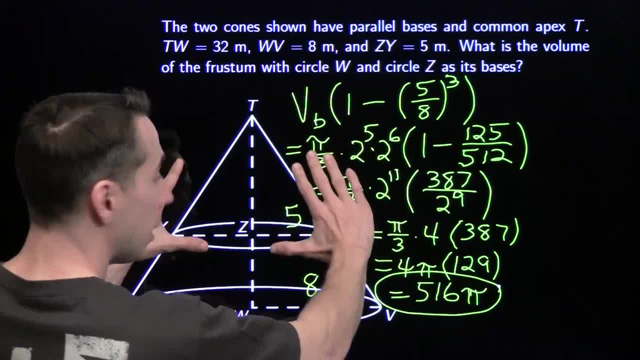 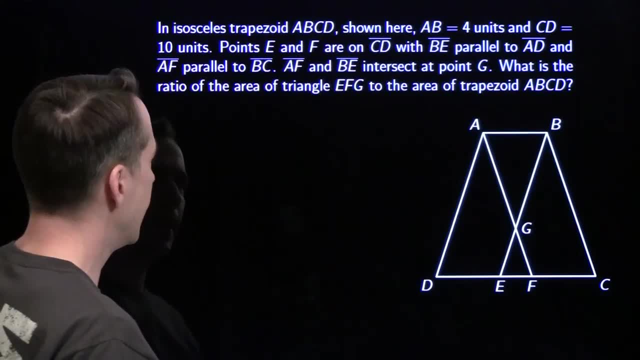 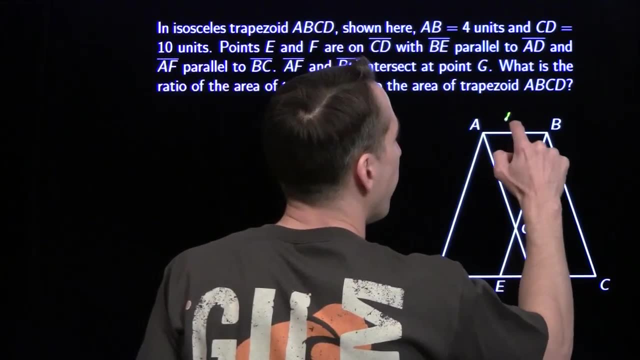 You just think of your frustum as a big cone with a little cone chopped off. On to the next problem: Trapezoid, Isosceles, trapezoid, AD, BC are equal. Let's see AB is 4.. 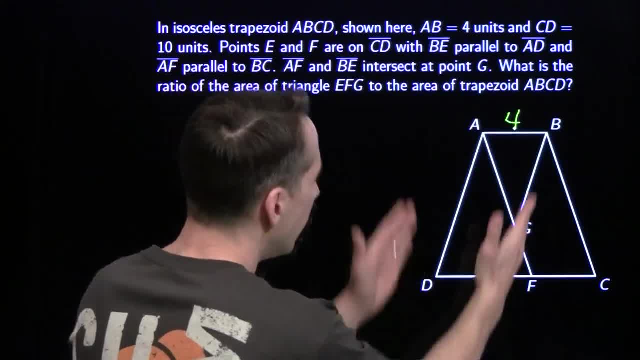 CD is 10.. We've got ENF down here. BE is parallel to AD, AB is parallel to ED. This is a parallelogram. That's 4.. That means this is 4 down here. We've got the same game going on over here. 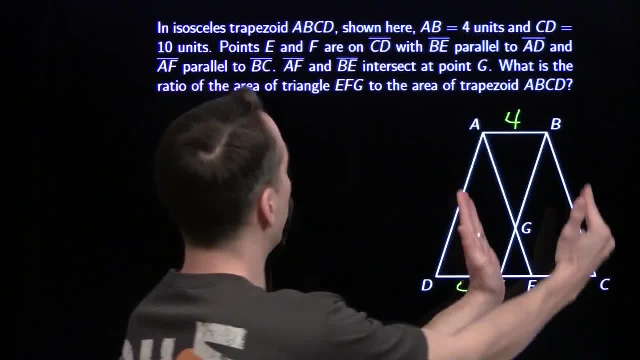 All right, We've got. AF and BC are parallel. This is a parallelogram. It tells us, this is 4. And we were told that this is 10. So this little piece is 2.. That's the arithmetic even you can handle, Harvey. 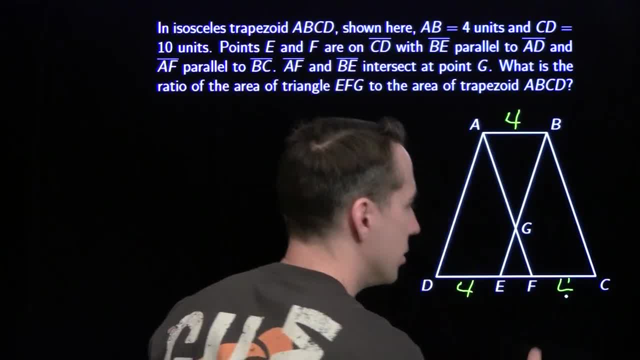 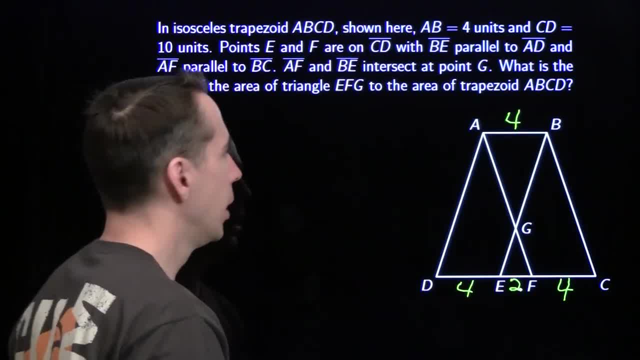 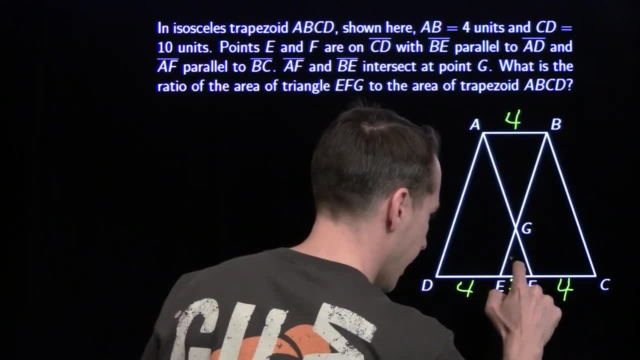 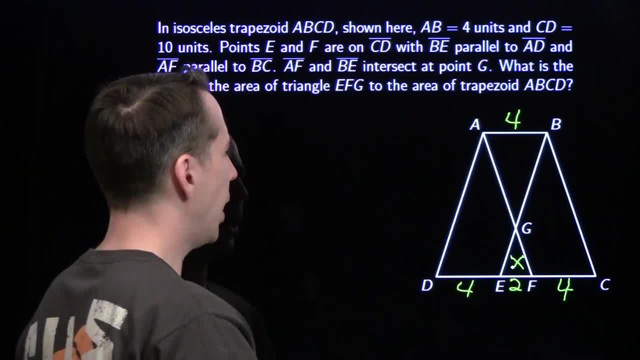 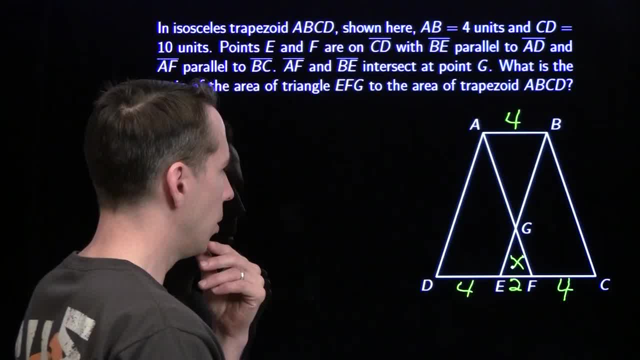 height. here I can make up a height and start cranking through, but that looks like work, So we're going to think a little bit first What I'll think back to now. Well, back here we used similarity to relate volumes. 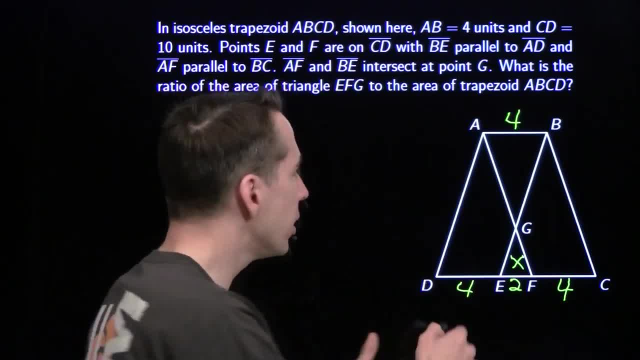 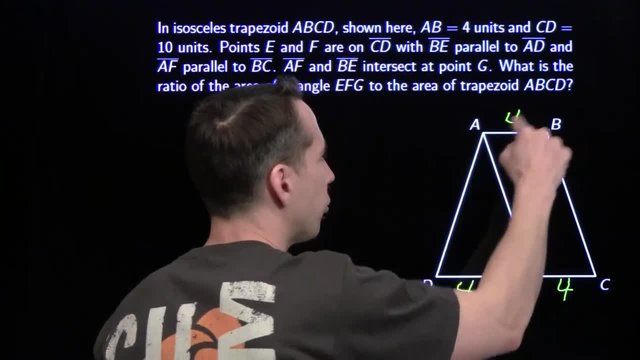 Well, here we can use similarity to relate areas. These two triangles are similar, So these two sides are parallel. Now the side lengths of this triangle are double the side lengths corresponding side lengths of this. So the area of this is 4 times the area of that. 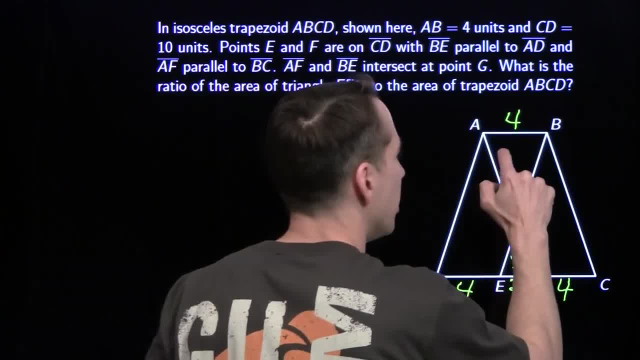 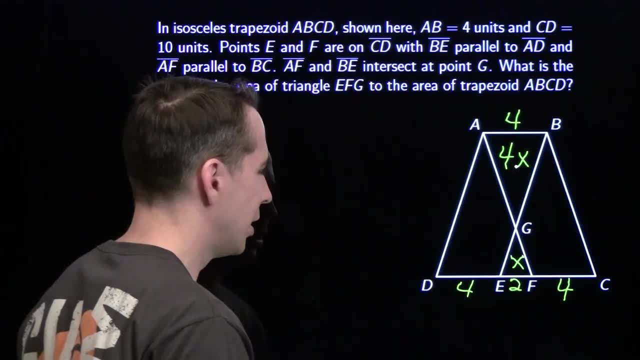 You just square the ratio of your side lengths to get the ratio of your area. So the area of this is 4x. but now we've still got these out here. I'm still stuck. Do it again, Oh yeah. yeah, it's one of my favorite strategies, all right. 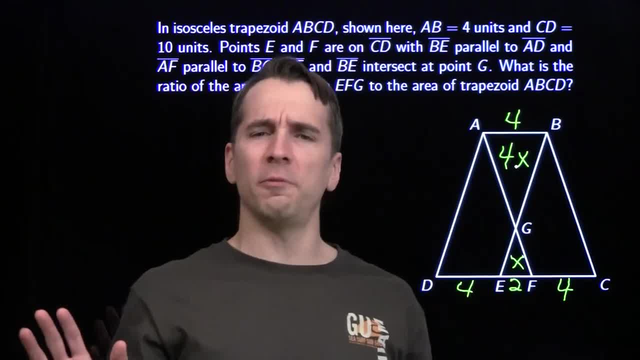 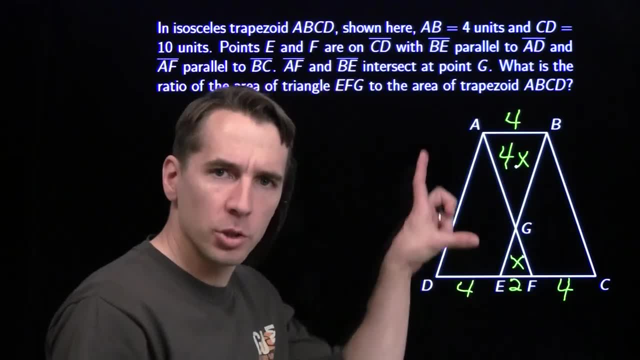 If you use something in a problem and it gets you a little bit out of the way but doesn't quite finish, try to immediately find another way to use that same strategy. Now, the strategy we used here was looking at similar triangles and relating their areas. 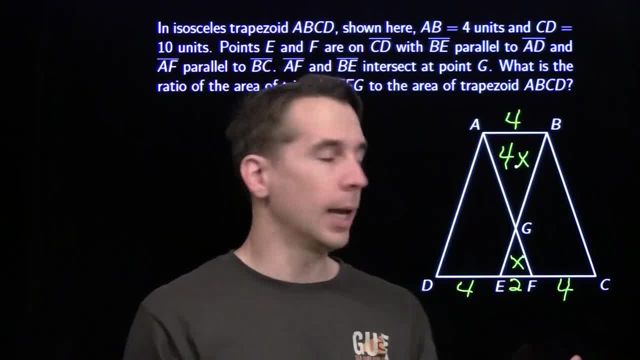 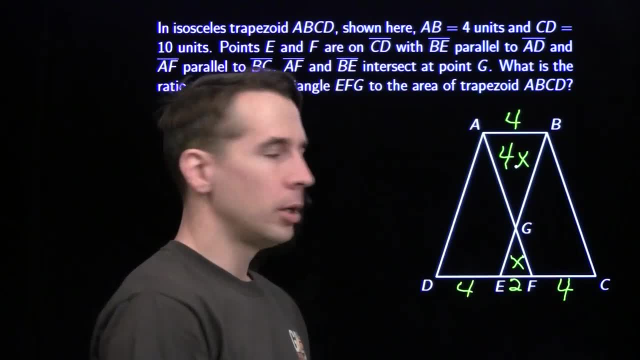 We've got lots of parallel lines in this problem. Maybe we can do it again. Look at these parallel lines. These parallel lines tell us that this triangle is similar to this triangle, So we can relate the area of BEC to the area of GEF. 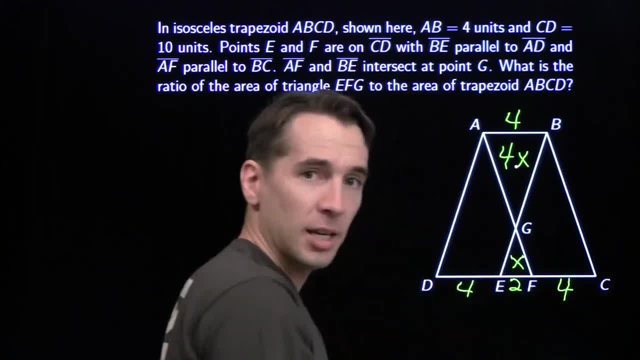 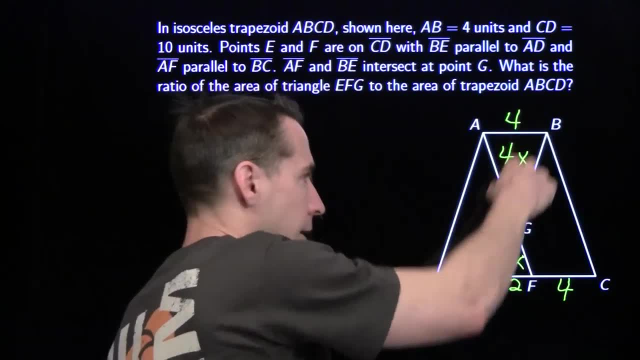 Now this side length is 2.. This whole side length is 6.. So the sides of the large triangle are 3.. That's 3 times the size of the small triangle. So that means the area of the large triangle is 9 times the area of the small triangle. 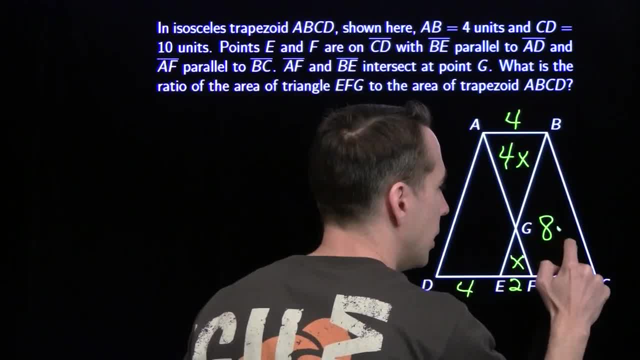 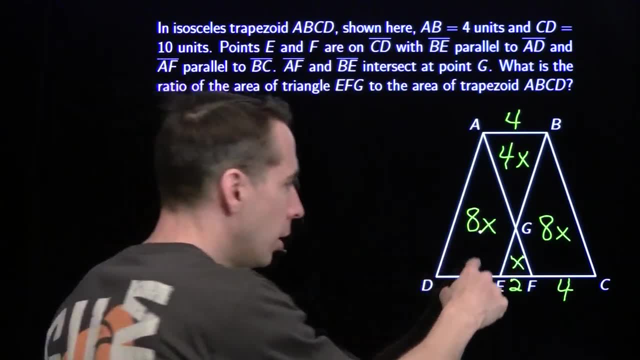 The whole thing right here has to be 9x. That means this piece is 8x and this piece will be 8x too, because we've got the same thing going on over here And now you're all set. 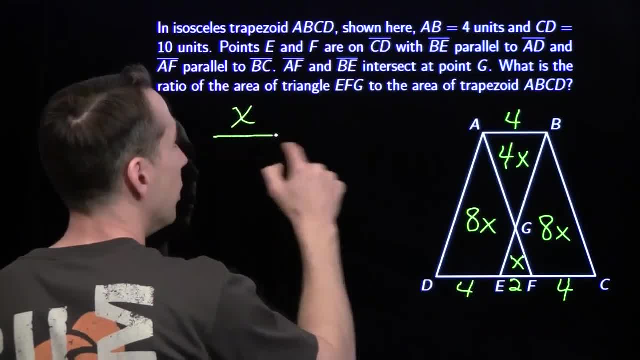 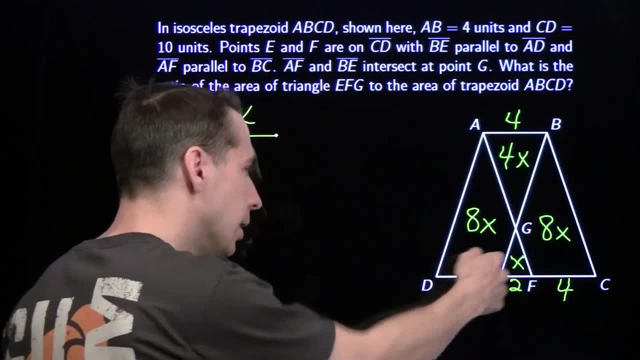 Little triangle area is x, and then the entire trapezoid ABCD. we just add this all up: 4x, 8x, that's 12.. 12 and 8 is 20.. That one more we got. 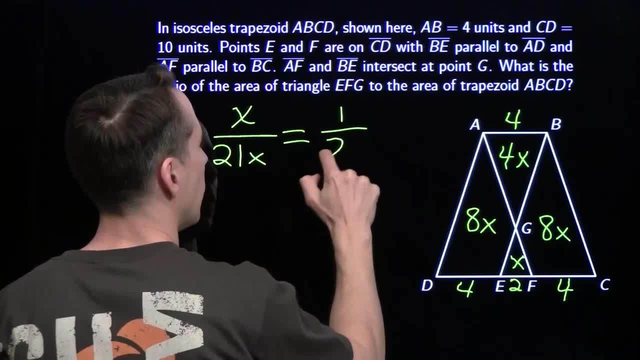 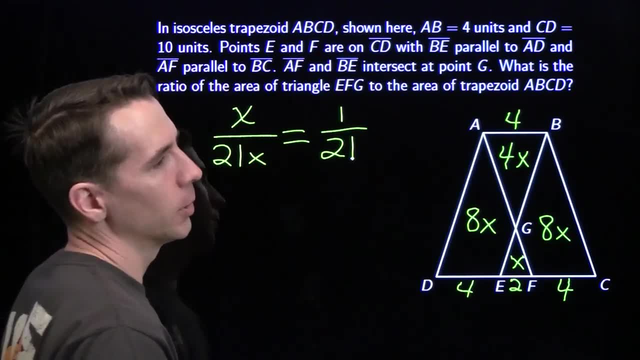 x over 21x gives us 1 over 21.. Long way I knew you were going to say that I knew it. All right, what's the short way, Harvey? Think about the frustum. What's a frustum? 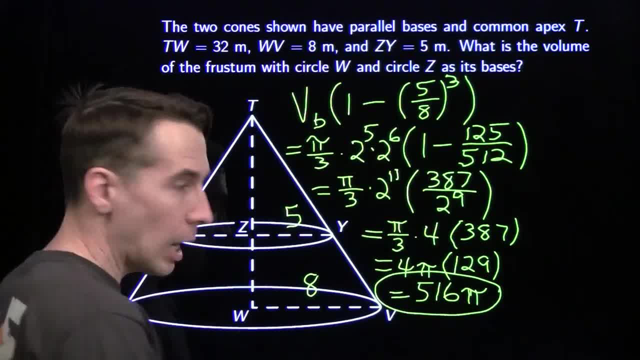 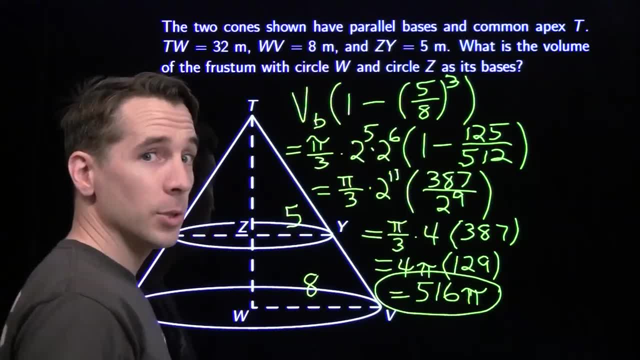 A frustum is just a. Okay, I'll say it again: A frustum is what you get when you chop the little cone off the big cone. Base is parallel and da-da-da-da, What's a trapezoid? That's what you get when you chop a little triangle off a big triangle. 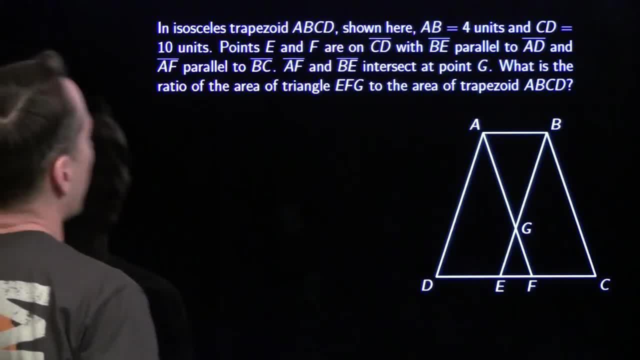 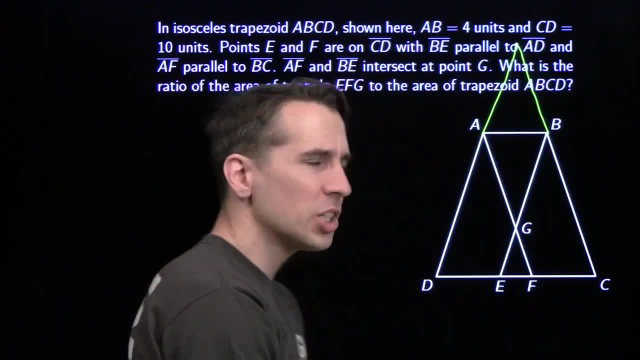 Let's try that, All right. so we got another look at a trapezoid here. Here's our trapezoid. We're going to think of this trapezoid as what we get when we chop this little triangle up here off the big triangle down here. 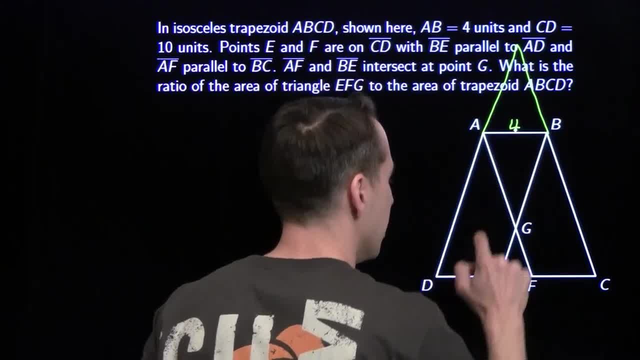 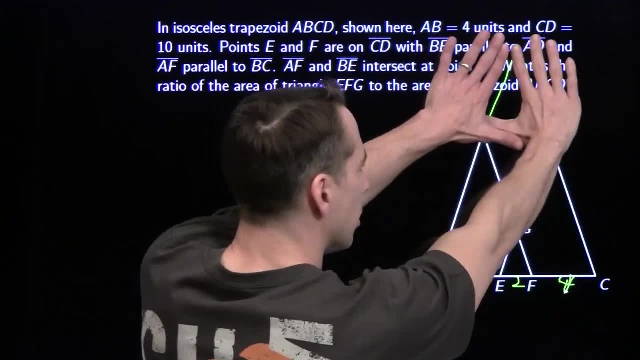 How does that help? Well, we were told that I'll go ahead and put in these side lengths again. This was 4.. This is 4.. This is 2.. This is 4.. All right, So this piece up here. I got the parallel lines. 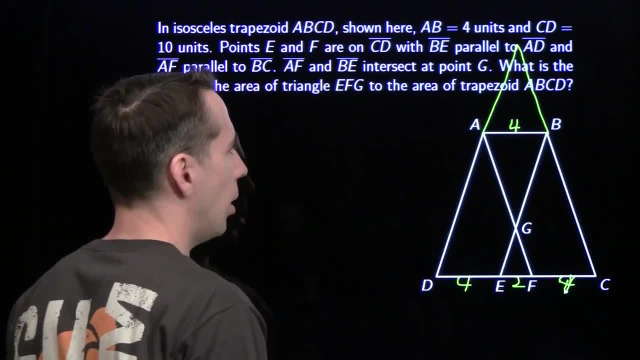 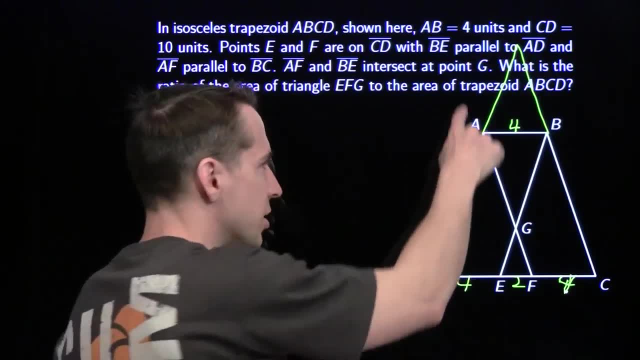 This piece is similar to this piece And so this piece up here its side length is 4.. This one's 10.. So this, the side lengths here are 2 fifths the side lengths of the big triangle. That means this area is 4, twenty-fifths of the whole thing. 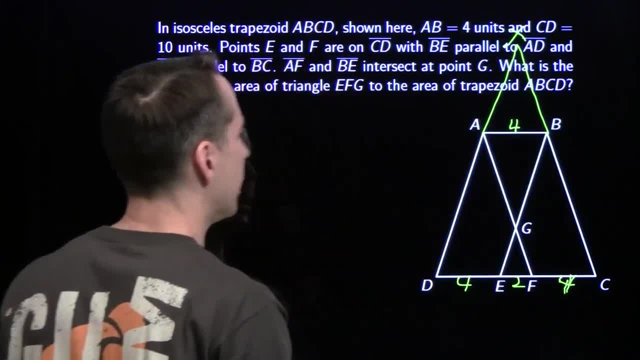 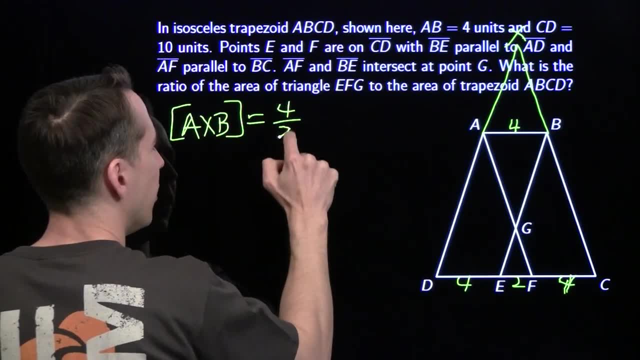 So I'm going to write that. let's see, we're going to call it like that. We're going to go AXB. I'm going to put brackets to mean area. It's 4, twenty-fifths, 4, twenty-fifths, the whole thing, the big triangle which is DXC. 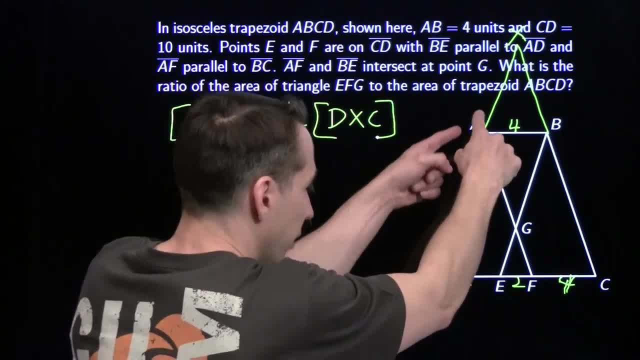 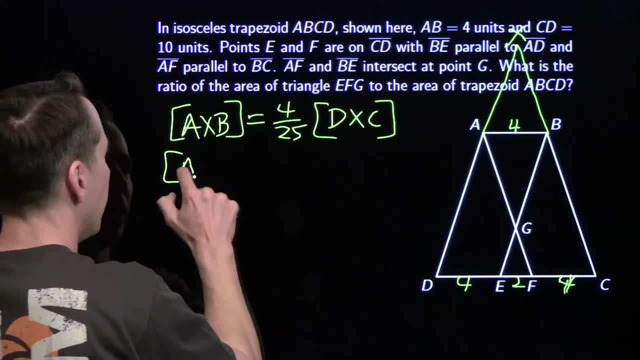 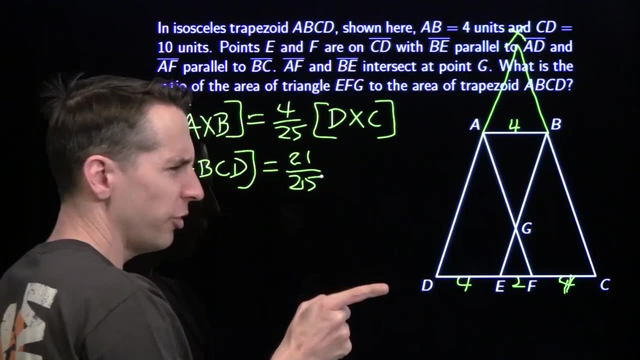 All right, well, that tells me. that leaves the trapezoid. there is what's left from the whole thing. You have the whole triangle minus 4 twenty-fifths of the whole thing. That tells me that ABCD is 21- twenty-fifths. oh, there's that, 21.. 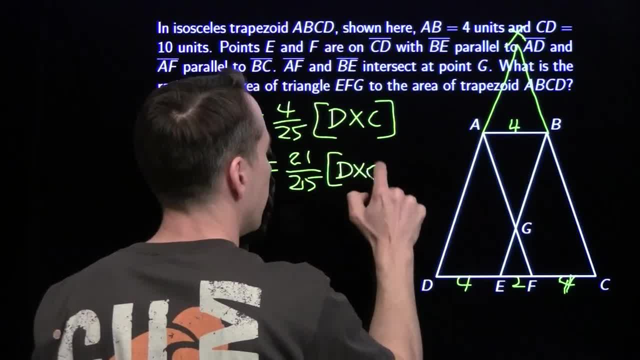 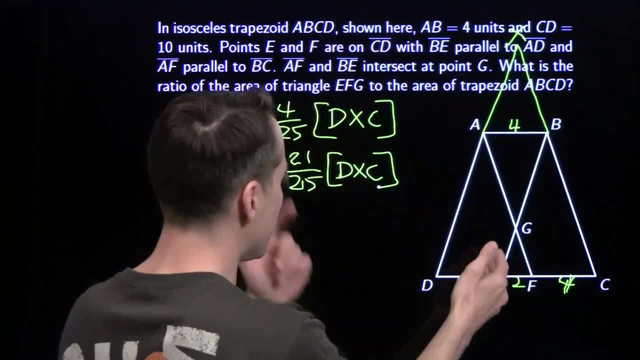 You're sneaky of the whole big triangle. And then We've got more similar triangles, The little triangle right here. from the very beginning of the problem, this EFG is similar to the big triangle. Its side down here is 2.. 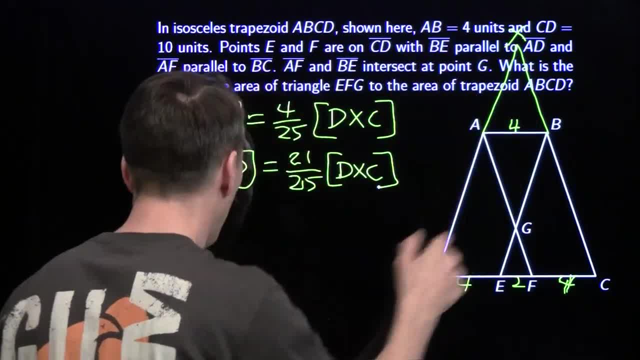 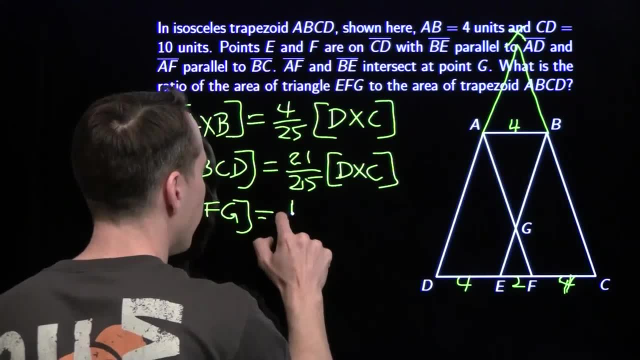 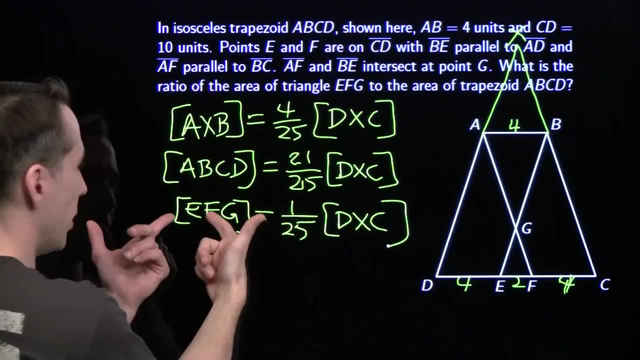 This whole thing is 10.. So its side lengths are 1 fifth out of the whole triangle. So its area is the square of 1 fifths is 1 twenty-fifth of the entire big triangle. And there we go. The ratio of this to this.